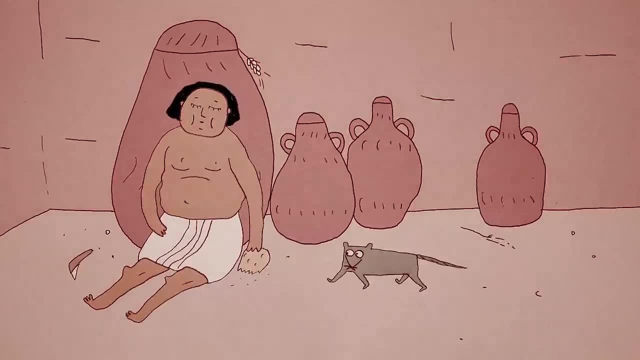 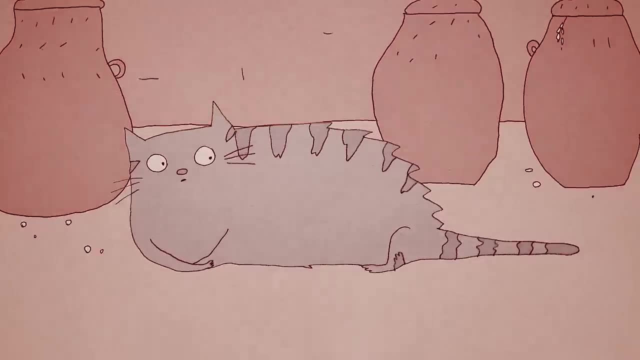 They stored their excess grain in large pits and short clay silos, But these stores of food attracted hordes of rodents, as well as their predator, Felis sylvestris libica, the wildcat found across North Africa and Southwest Asia. These wildcats were fast. 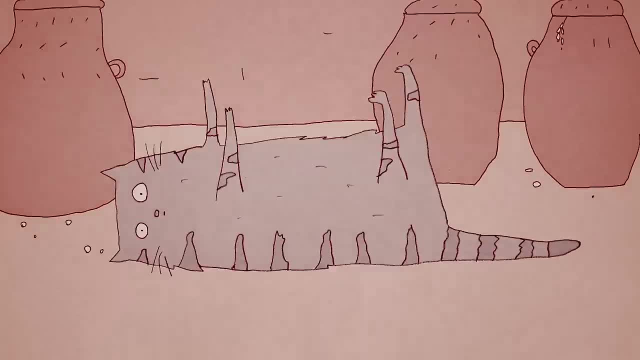 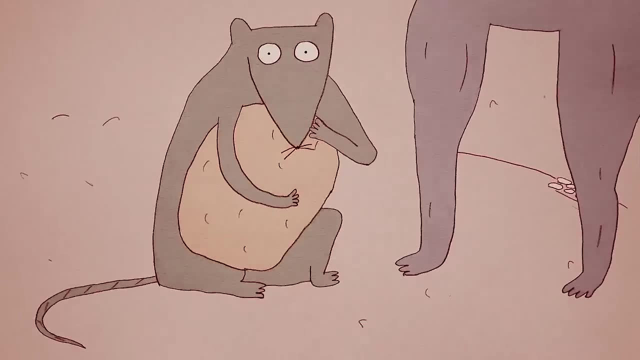 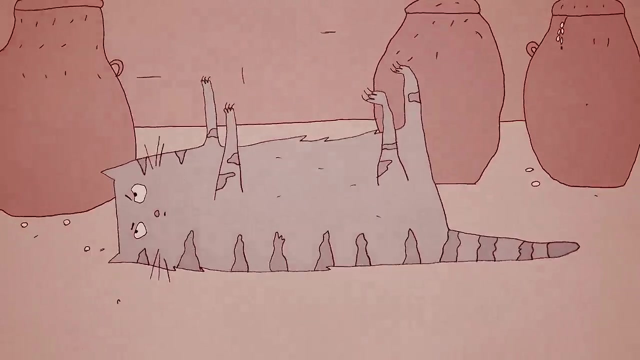 fierce carnivorous hunters, and they were remarkably similar in size and appearance to today's domestic cats, the main differences being that ancient wildcats were more muscular, had striped coats and were less social towards other cats than humans. The abundance of prey in rodent-infested greeneries drew in these typically solitary 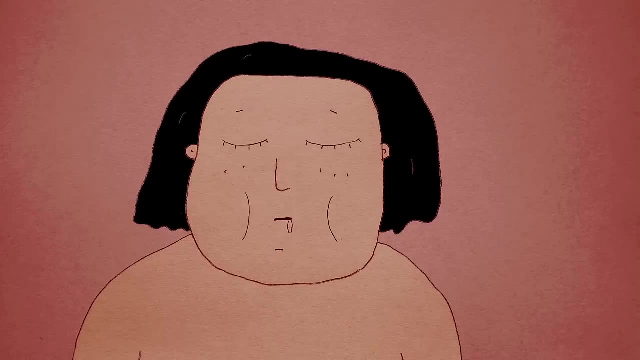 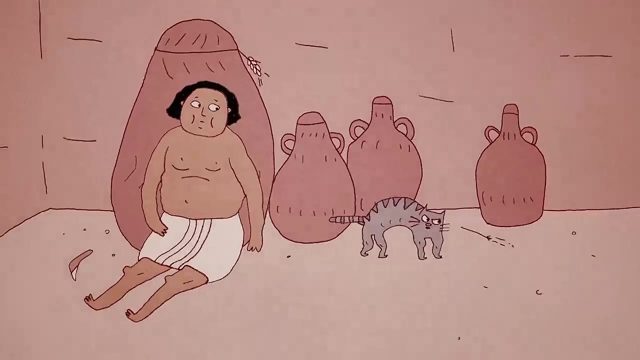 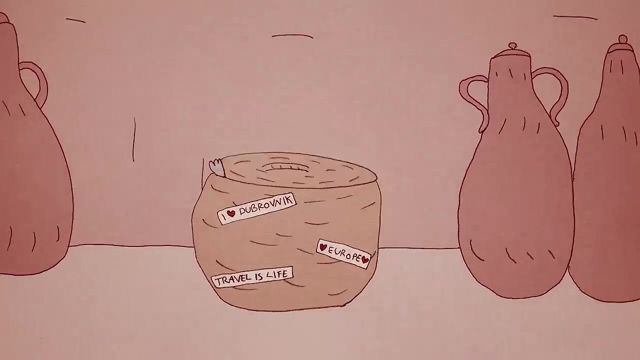 animals, And as the wildcats learned to tolerate the presence of humans and other cats during mealtime, we think that farmers likewise tolerated the cats in exchange for free pest control. The relationship was so beneficial that the cats migrated with Neolithic farmers from Anatolia into Europe and the Mediterranean Vermin, were a major scourge of the Seven Seas. 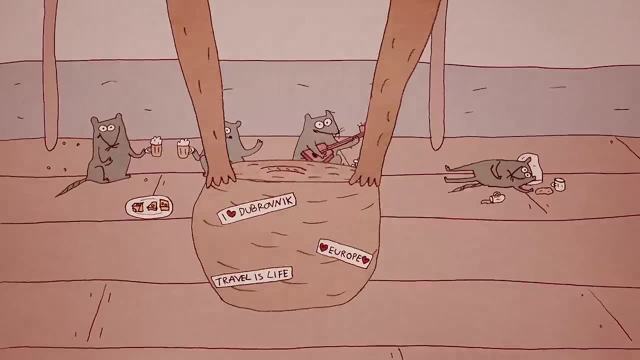 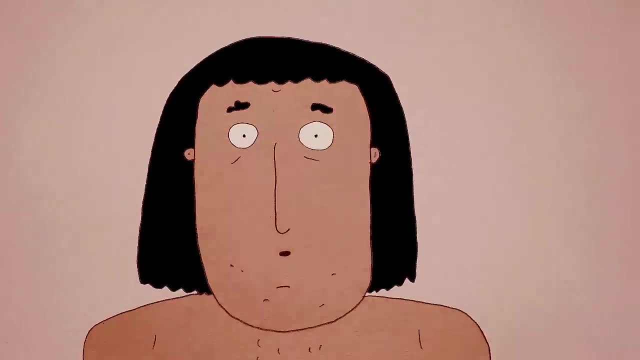 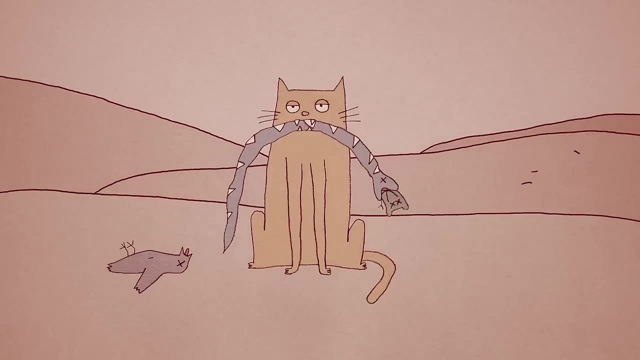 They ate provisions and gnawed at lines of rope, So cats had long since become essential sailing companions Around. the same time these Anatolian globetrotting cats set sail, the Egyptians domesticated their own local cats, Revered for their ability to dispatch venomous snakes, catch birds. 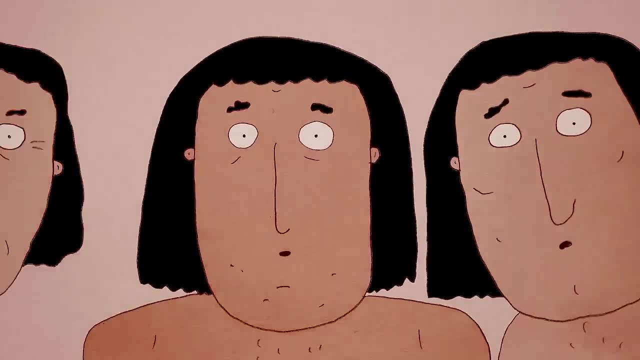 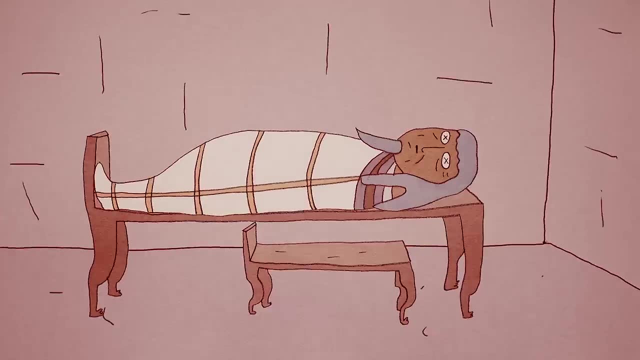 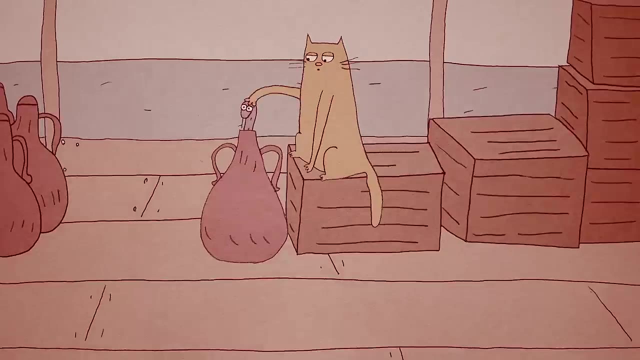 and kill rats. domestic cats became important to Egyptian religious culture. They gained immortality in frescoes, hieroglyphs, statues and even tombs mummified alongside their own owners. Egyptian ship cats cruised the Nile holding poisonous river snakes at bay And after graduating. 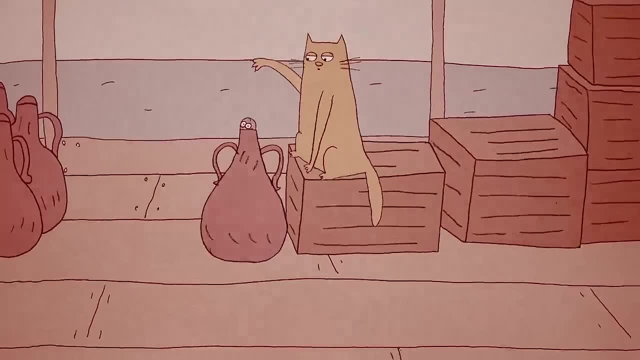 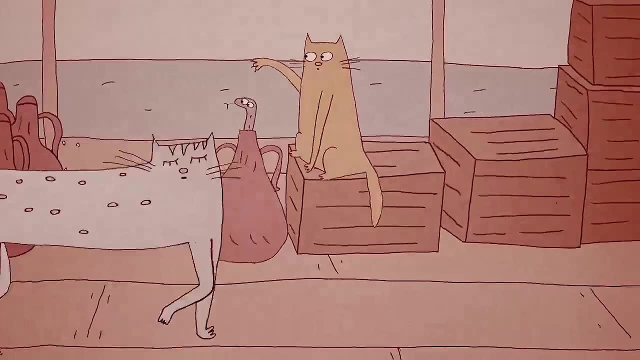 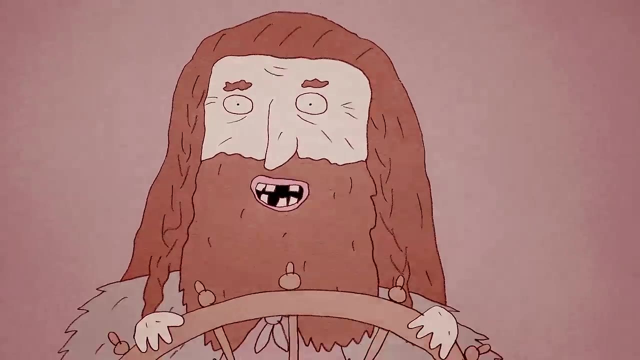 to larger vessels. they too began to migrate from port to port During the time of the Roman Empire. ships travelling between India and Egypt carried the lineage of the Central Asian wildcat FS ornata. Centuries later, in the Middle Ages, Egyptian cats voyaged up to the Baltic Sea on the ships. 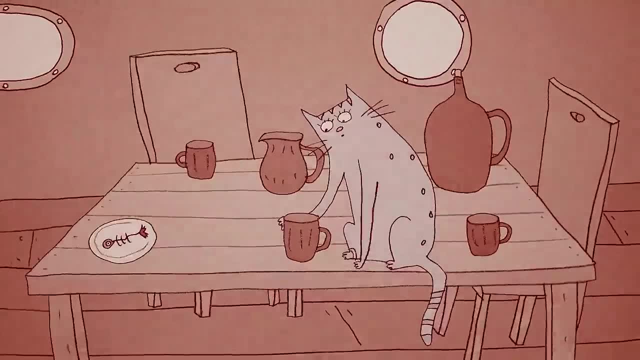 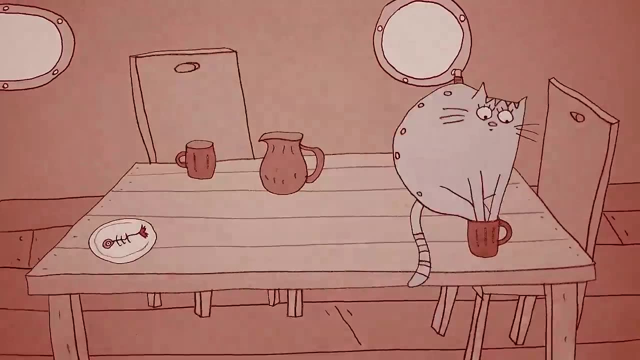 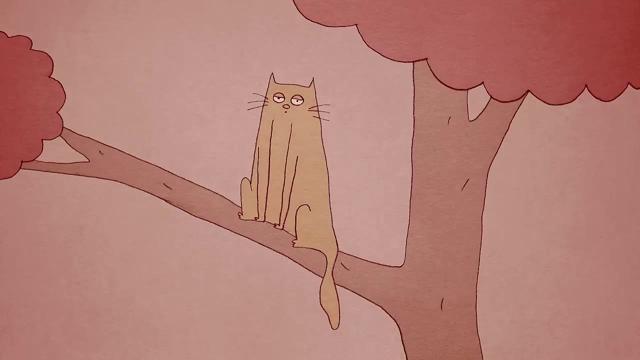 of Viking sea-fairies And both the Near Eastern and North African wildcats probably tamed at this point, continued to travel across Europe, eventually setting sail for Australia and the Americas. Today, most house cats have descended from either the Near Eastern or the Egyptian lineage.